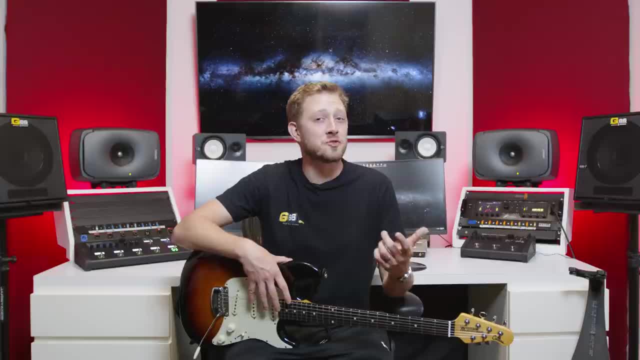 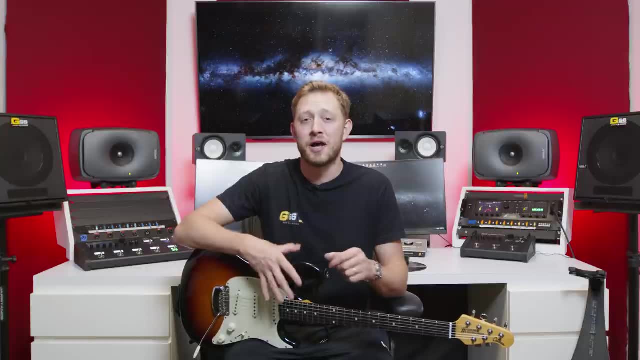 their time jamming out alone. these three tips are going to help you. So if you're a player that's looking to sit perfectly in a mix and really shine in that spot, here are three very quick, very easy tips that'll thread the fine needle of making you cut through the mix stand. 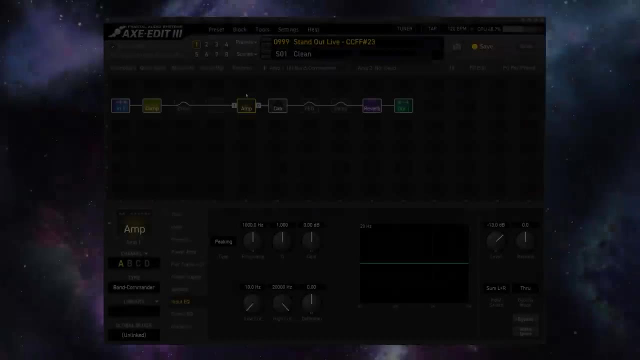 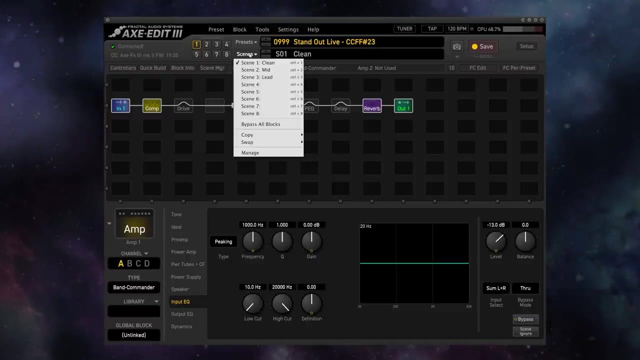 out but also meld seamlessly with the band. Okay, so we're going to start off with a simplified version of my go-to live preset. I've got three scenes: a clean, a mid-gain and a lead. So here's. 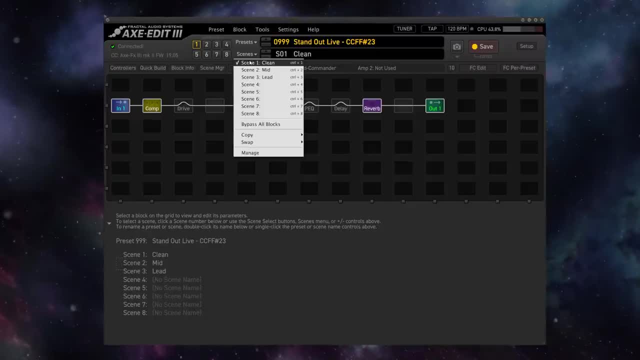 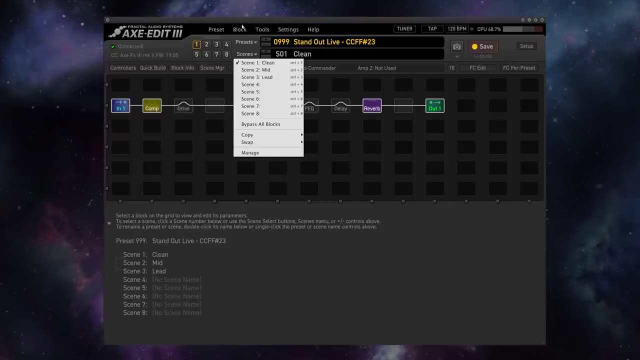 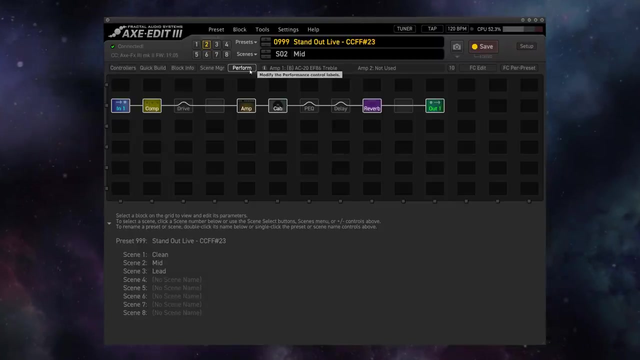 the clean. Here's the clean. Now. those are three great tones to me, but the front-of-house engineer would probably do a lot to those tones to make them ready to sit in a mix. Now where I'm sitting right now, in my 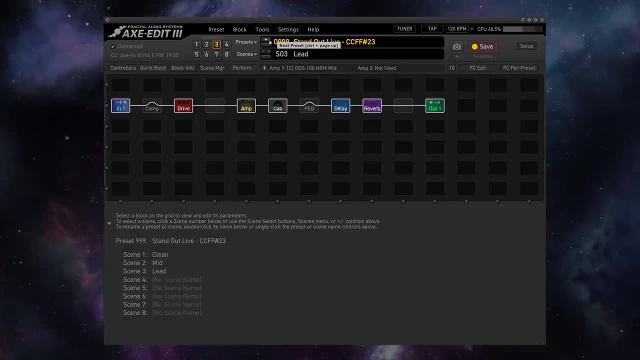 studio playing alone with my full-range speakers cranked way up. I'm very satisfied with these tones, But there is, admittedly, a lot of bass content and a lot of high-end content that really doesn't need to be there, And you can see that if we put a real-time analyzer block. 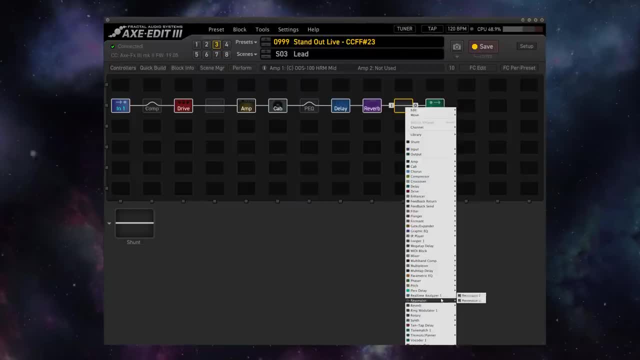 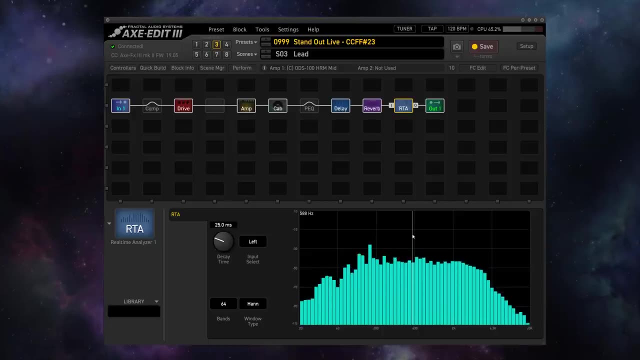 in our preset. here I'm going to just add the RTA and we can play and you'll see There's a lot happening below 100, and there's a lot happening above 6k. that really is just going to be interfering with the cymbals and the kick drum and the bass guitar. 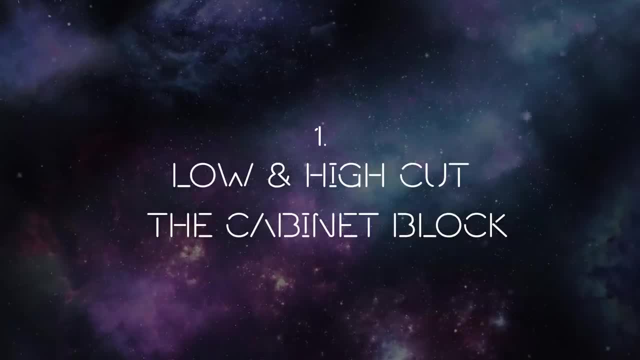 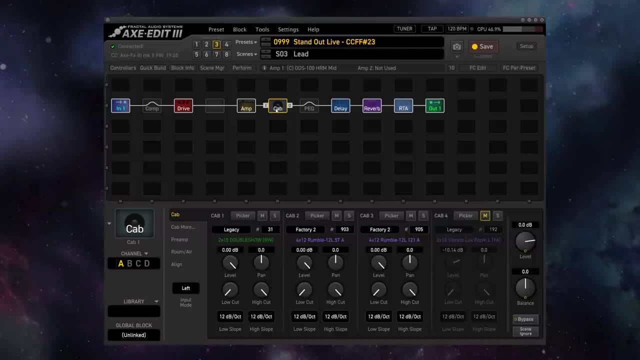 So the first thing I do to every tone that I take out live is to low-cut and high-cut the cabinet block. Now, the benefits of this are twofold. Number one: if you're going into a PA, you're going to make the guy at front-of-house really happy because 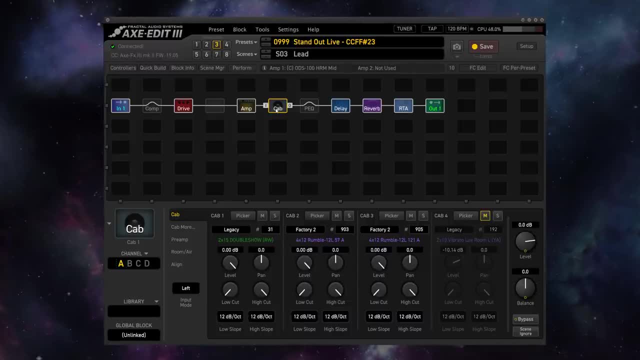 he may not even have to do any EQing at all to your tone to get you to sit really nicely in the mix. The second benefit, which may be even bigger for a lot of players, is that if you are gigging with only an FR-FR speaker on stage, so a full-range flat-response speaker instead of an amp. 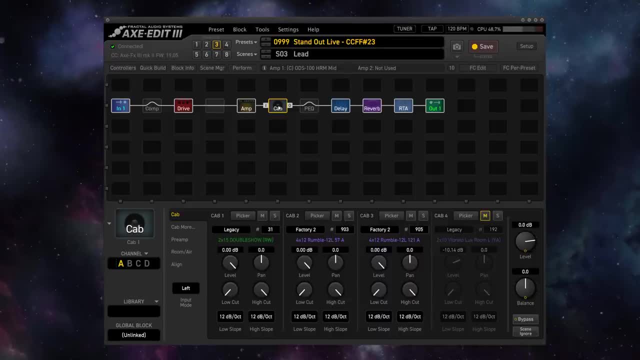 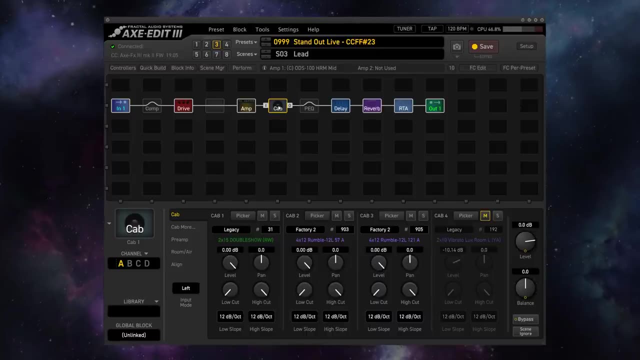 if you're playing like a club gig or a bar gig and that is your only sound- low-cutting and high-cutting- that FR-FR is going to get you sitting perfectly in the mix. I hear from so many players who say they have dialed in a perfect tone in their rehearsal space and then when they get 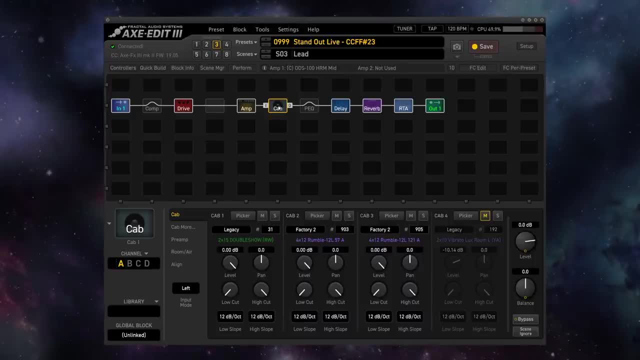 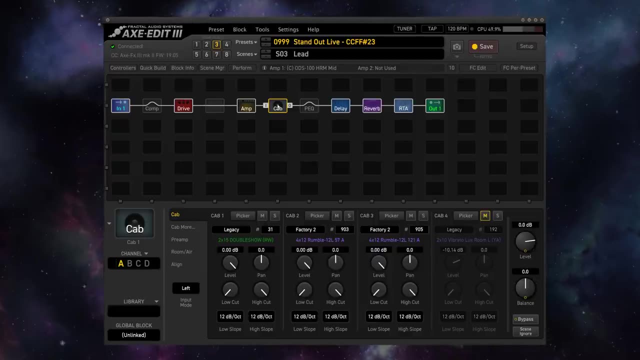 to the gig. they're lost in the mix, playing onstage with just their FR-FR, And that is likely because you're not低-cutting and low-cutting their tones sufficiently so that the band versus the guitar becomes a volume more and everybody keeps turning up to try. 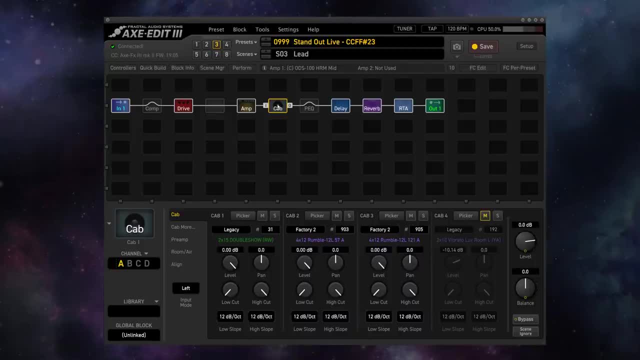 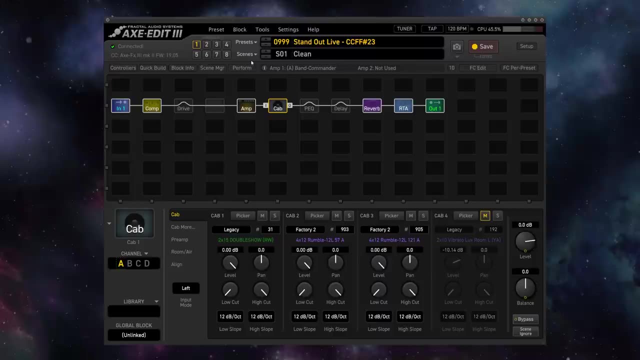 to make their parts cut and then it turns into a giant muddy mess. So again, right off the bat, first thing I do for live tones is I go into the cabinet block- We're going to start with scene one on cabinet channel A- I go into the preamp and I'm going to use these low cut and high cut. 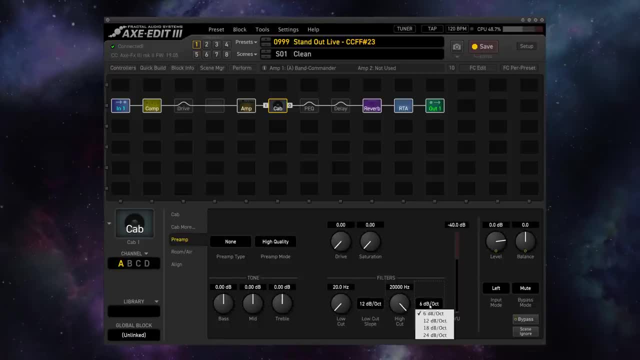 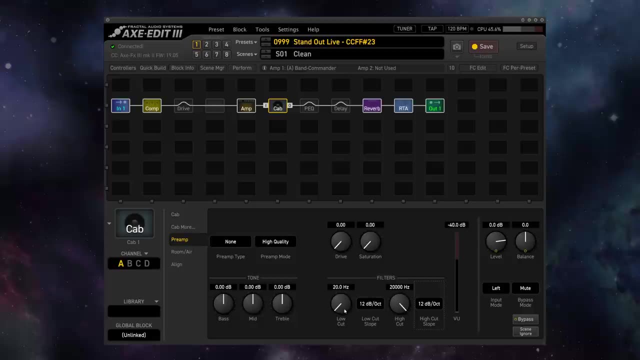 parameters. So first off I'm going to set the slope to 12 dB, so I've got a little bit steeper slope on my filter, and then I'm going to low cut anywhere from 50 to 120 hertz, and this is. entirely up to you and may depend on what you're monitoring through and really can change depending on what kind of tone you're dialing in. I generally find myself getting around 80, and that's where I like to start. 120 can be really aggressive for a lot of tones, but for some higher gain tones. 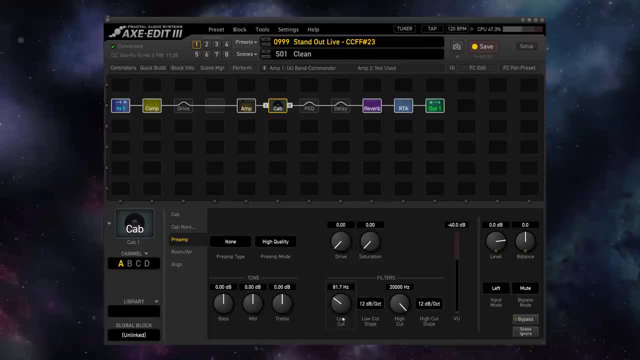 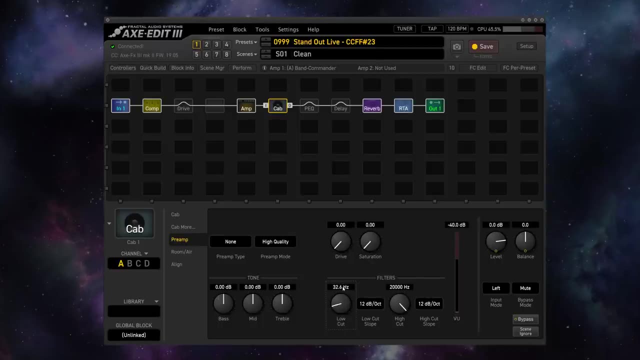 that can be right where you want for the tone to sit. So let's hear the clean Clean here without any low cut at all, And then turning the low cut up to about 80 here. Now you can hear that the core of the tone is very much still there. It really does not sound. 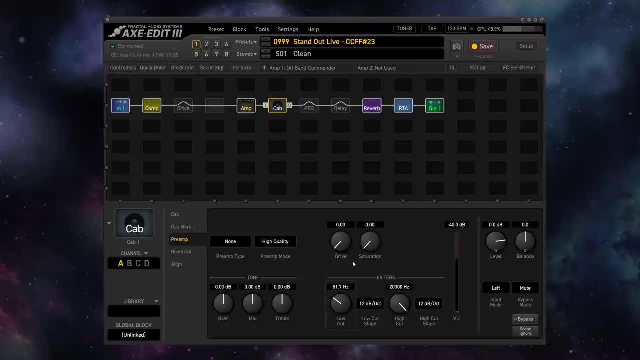 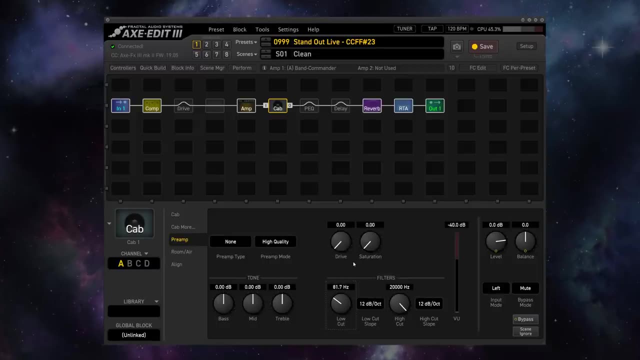 a whole lot different and, in fact, if you're listening on a phone or on a tablet, you may not hear any difference at all. I encourage you guys, as with all of my videos, to listen on the best speakers you can and listen at a pretty loud volume to really hear what I'm hearing here in. 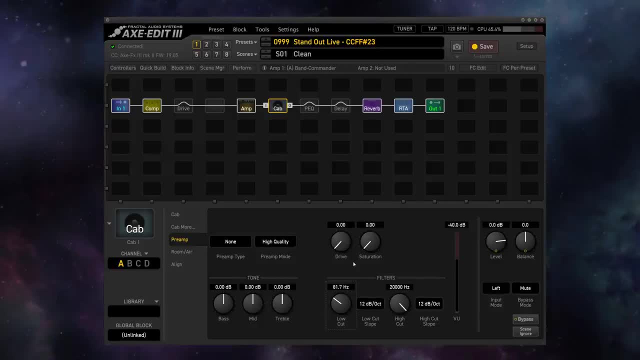 the studio. So next up we're going to high cut and again, this is entirely up to you and entirely up to the tone where you end up. Generally, you're going to want a high cut starting from anywhere about 5K. all the way up to 10K. I generally find myself living somewhere around 7.5.. So 7500Hz and that's going to give us this kind of tone. Yeah, Okay, Okay, Okay. 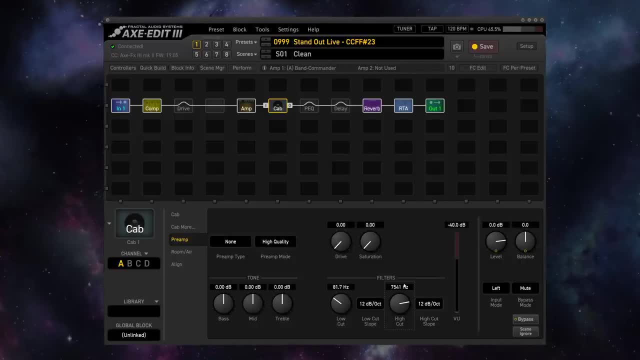 Okay, Okay. if you are following along and dialing in your own tone here, you may now feel like your tone has lost a little bit of the sparkle, a little bit of the life and a little bit of the air. that's an understandable perception, but again, this is the kind of thing that is going to get you. 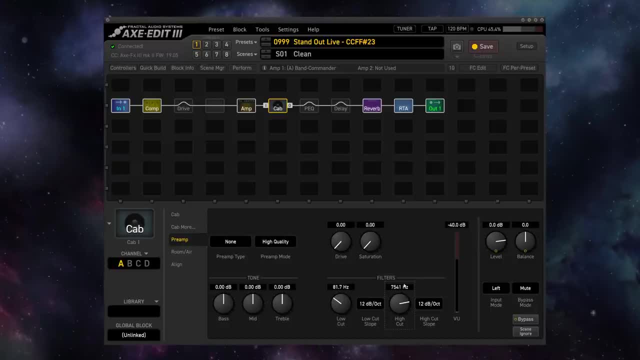 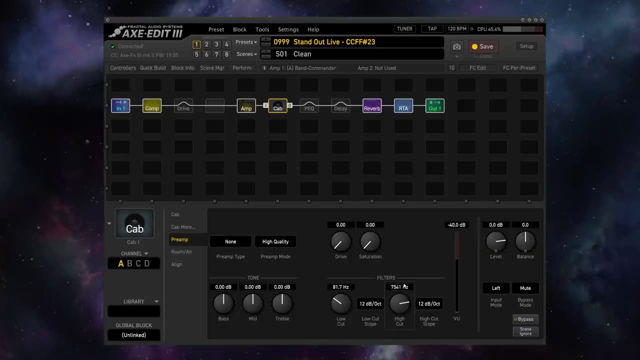 sitting better in the mix because your guitar is no longer going to be stepping on the other instrument frequencies up there in the high end. so for a lot of players, these kind of adjustments that you're used to not hearing because they're being made by front of house and only heard by 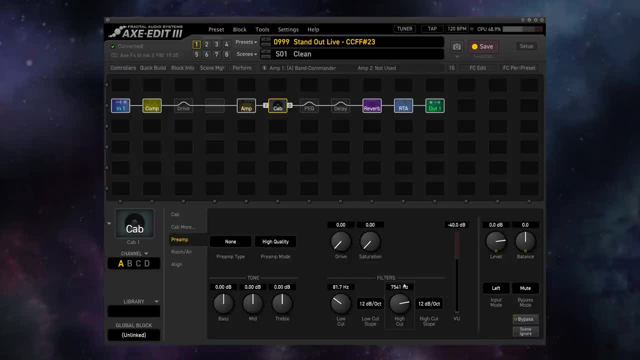 the audience can really be a lot to wrap your mind around, because you're used to hearing these tones that are taking up a whole lot of the sonic spectrum and sound a lot more pleasing to you. but i promise that if you make these adjustments you're going to find that your 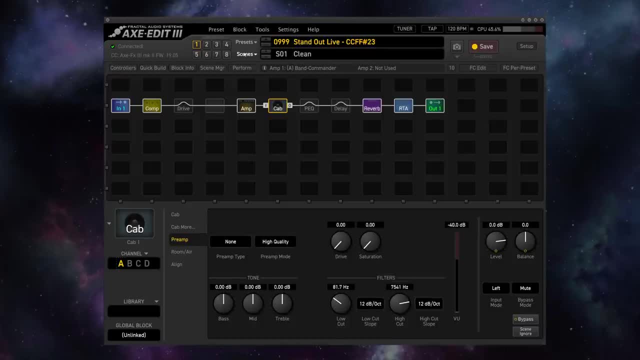 tones sit a lot better in the mix and you're going to be a lot happier. so i'm going to go ahead and move up to my mid gain, since i have a channel b in the cab here. so here's our tone again, and i'm going to go ahead and low and high, cut to the same values that i used before. 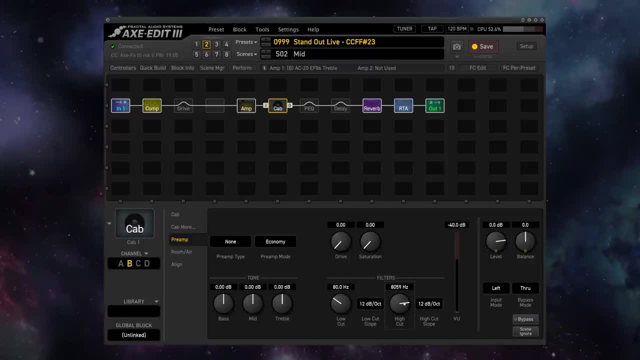 and i think for this tone i'm actually going to go ahead and raise this high cut up a little bit and bring this low cut down just a tad, and that's sounding a little better to my ears now. of course, these are the kind of settings that, if you have the benefit of dialing, 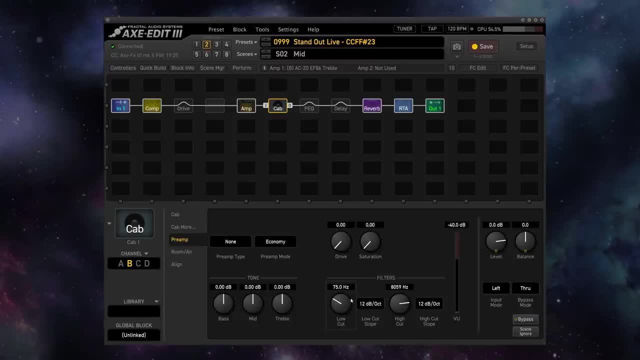 in while a band is playing or you're able to run backing tracks at the same time, you can really massage these values and take out a lot of the guesswork. i'm going with values that i know work for me, but again, there are wide ranges here that you guys can use. and now, if i go up to my lead, 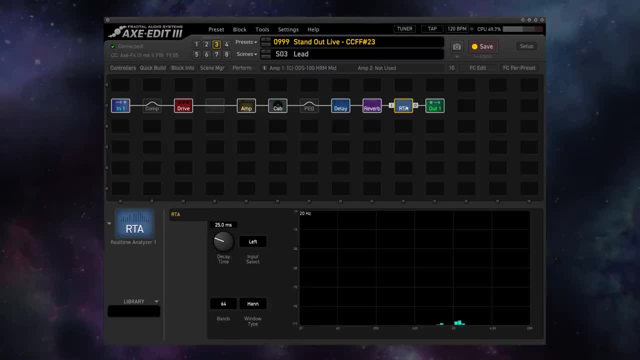 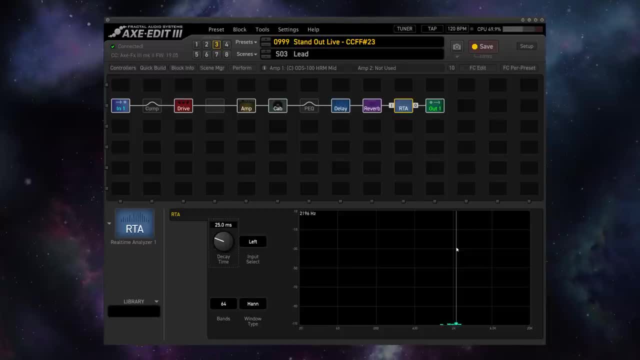 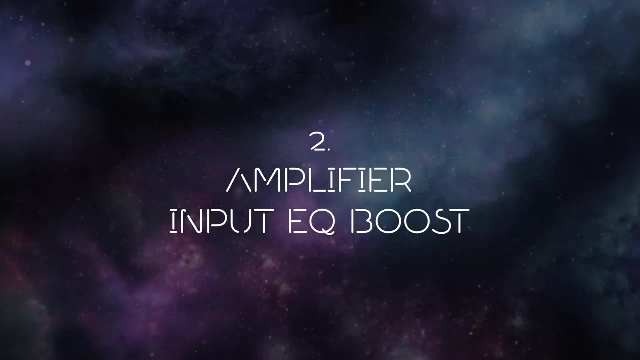 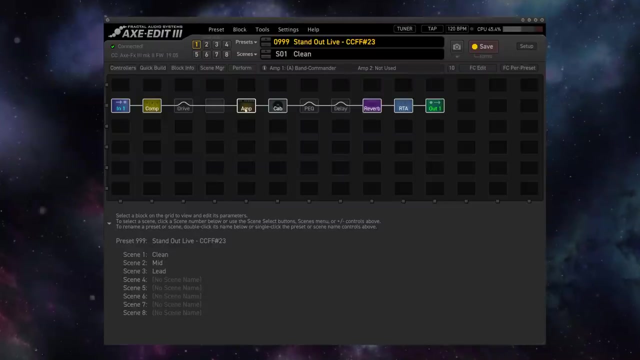 and you can really see how the curve and the slope of those low and high cuts are affecting the tone. much less information happening over here and over here. i have probably used this second little eq trick more than any other trick in the axfex or fm9 or fm3 and we find it in the input eq page. 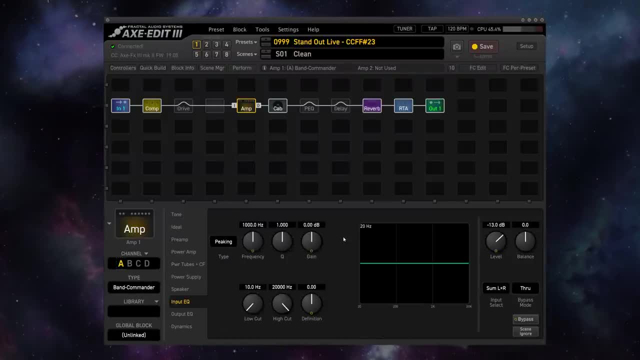 of the amp block. now the input eq page of the amplifier is a really nice way to affect the character of the amp and the tone of the eq on the amplifier. so i'm going to go ahead and go ahead and and i like to think of changes made here in terms of how the amp is speaking in the eq spectrum, as 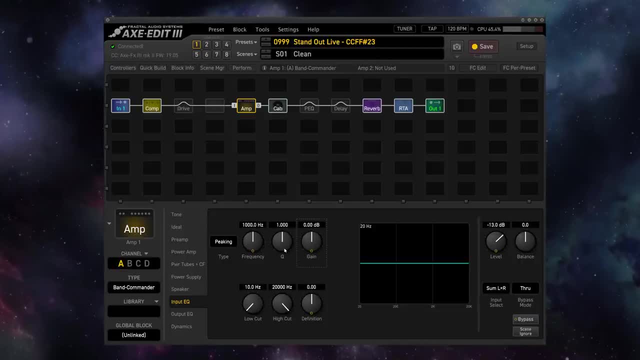 opposed to where. now, this trick is very straightforward, in fact. we can leave the frequency where it is, although you may find useful values between 900 and 1250.. we can leave the q where it is, on one, and i'm just going to take the gain up by about 3 db. now, again, you may find different values work for you and you can try experimenting with anything up to 6, although i find that a little aggressive. but let's hear the tone without this little gain boost at 1k and then i'll crank it up to 3 db and you can hear how this instantly adds a lift and a. 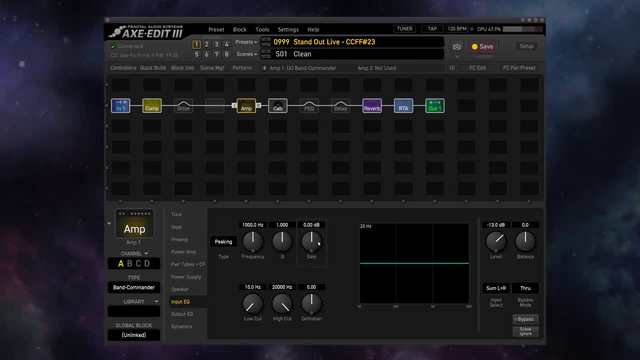 little bit of sparkle to your tone. i love what that does. the tone- and again i put this on pretty much every live preset i use- it really adds a nice subtle cut and it really, just to me, makes the guitar feel a little bit better under your fingers as well. so i'm going to go ahead and 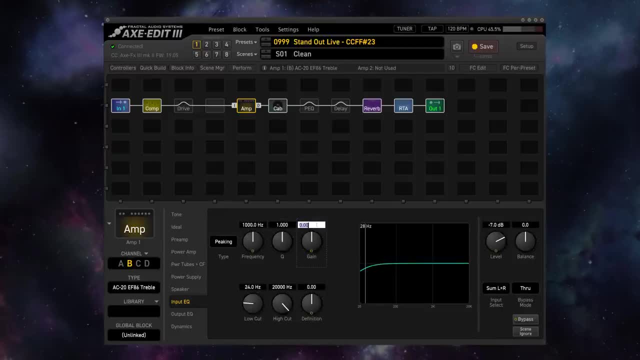 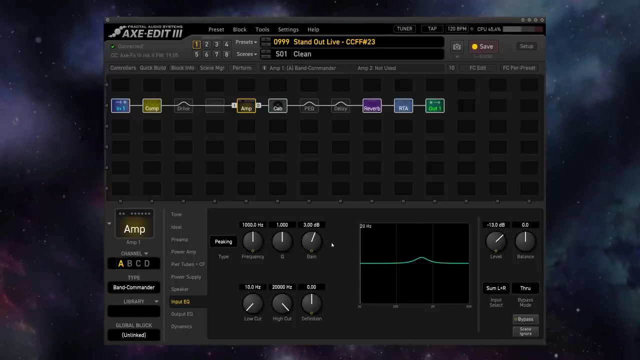 copy this into the other two amp channels here. i find this especially useful on leads, but again, i do generally add it to all of my tones. now, again, this is entirely up to you how much of this you want to dial in. i have used values as high as 6 db on this. but be careful: if you use a little too much of this it can start to sound. 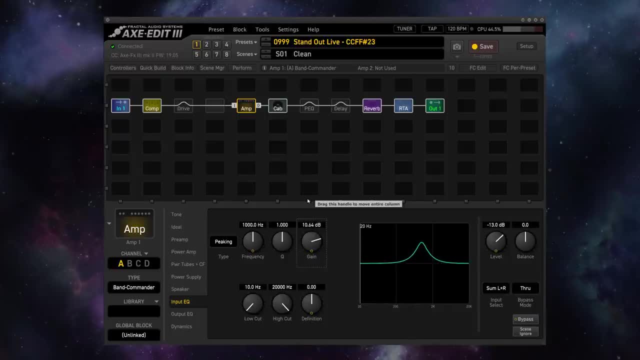 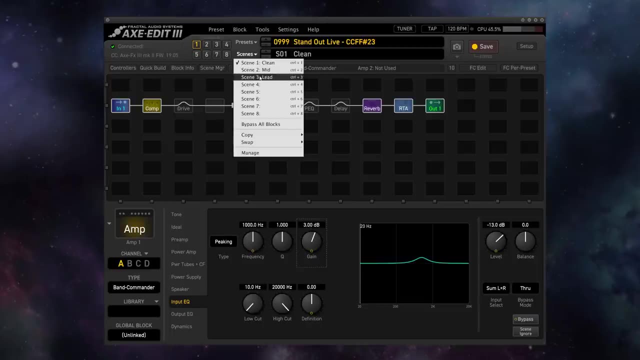 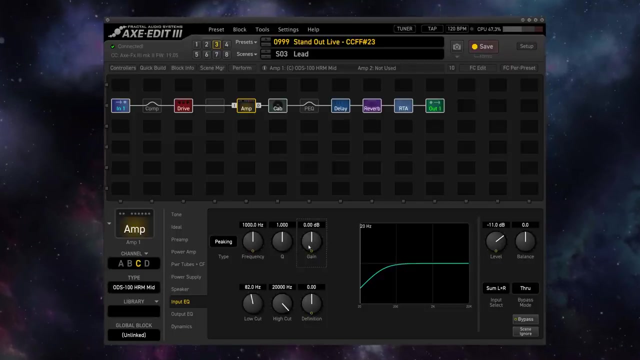 honky. so if i go ahead and crank this up, it can start to sound kind of unpleasant, so i'm going to put this back down to 3 db. let's listen to our lead, especially with this. here we are without the boost, so this to me feels like an instant cheat code to livening up your tone. 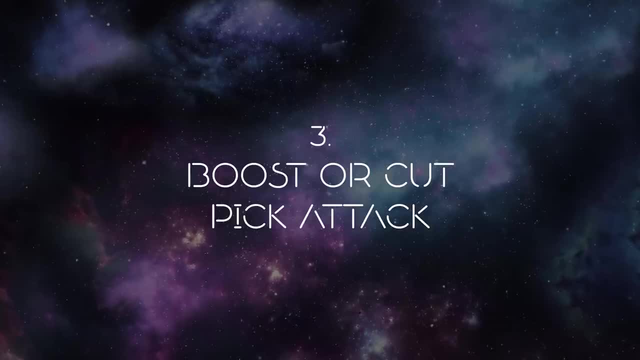 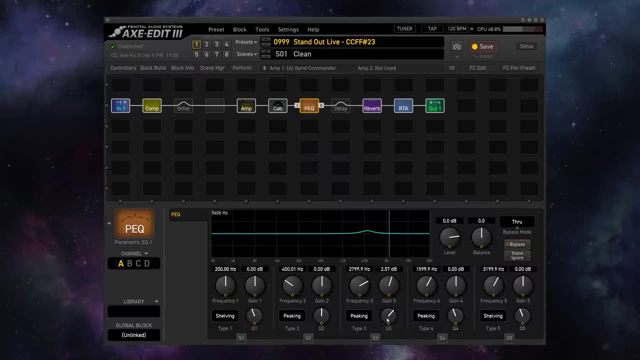 and finally, a quick trick using an actual eq block. i'm going to turn this guy on here and, as you can see, i've programmed a 3 db boost with a q of 2 right around 2800 hertz. now, between 2.5 and 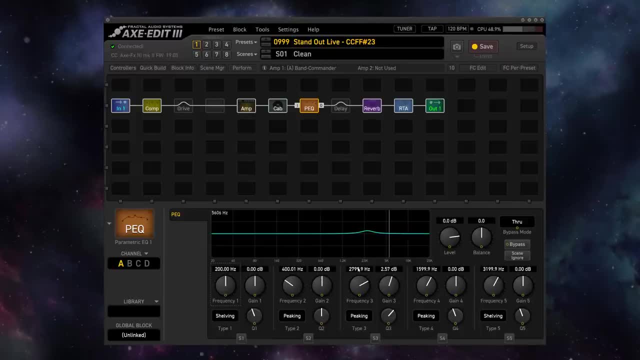 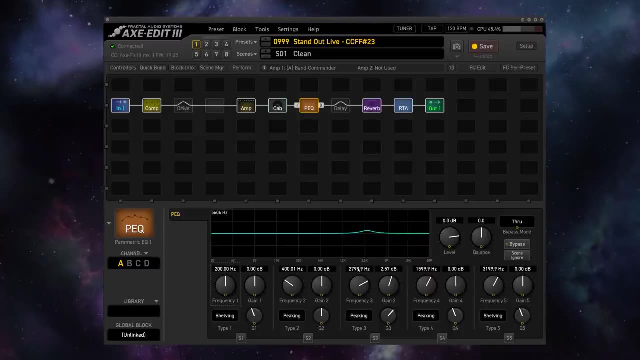 3k is really where a lot of the pick attack and the trans is going to be going to be going to be also have an additional boost level here. uh, so you can agitate your pick attack by using once from a сиг. you'll have this hugeção where the 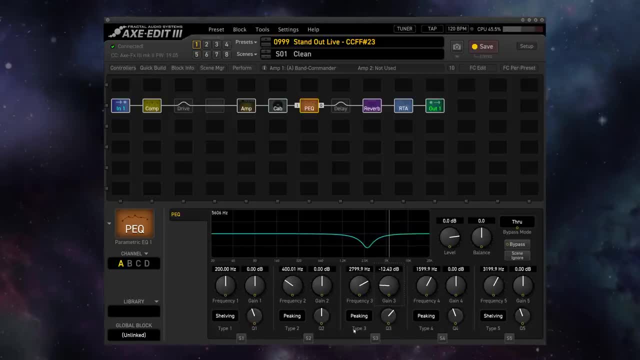 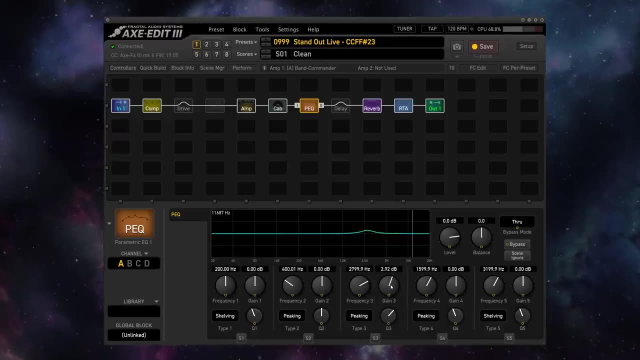 two transients of the guitars live, and so by either boosting or lowering this frequency range we can add or take away a pick attack. now, too much boost here and your tone will start to sound really shrill and ice picky, and too much taken away here can really bury your guitar in the mix because all of the pick attack and transients are gone. so adding a subtle lift here can really bring out pick attack, which can be great for tones where you're playing riffs or, for example%. 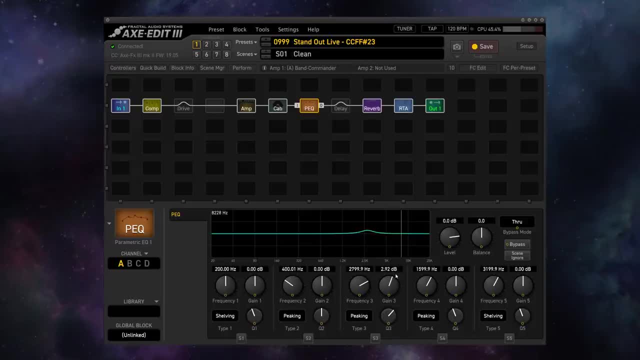 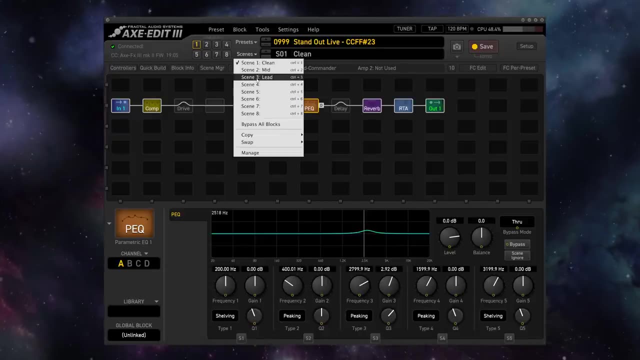 can set a speed limit with your cues and then increase the sound level and request new instruments to ourscheid, if you but cleans where you really want to hear the transients. And this can also be great if you're a shred type guy and you are doing a lot of alternate picking leads and you really want to. 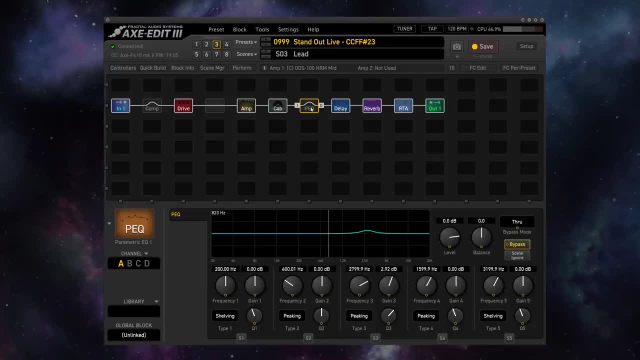 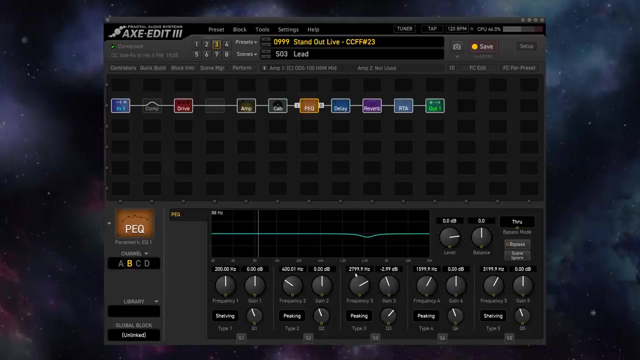 hear the pick attack. Now turn that coin over or, in this case, flip this curve over and we now have a gain reduction at 2800 and we are taking away pick attack, which can be really great for guys going for a Joe Satriani or Eric Johnson vibe, where you really don't want to hear as many transients. 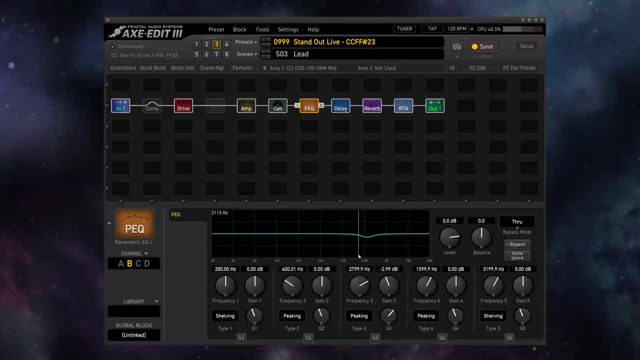 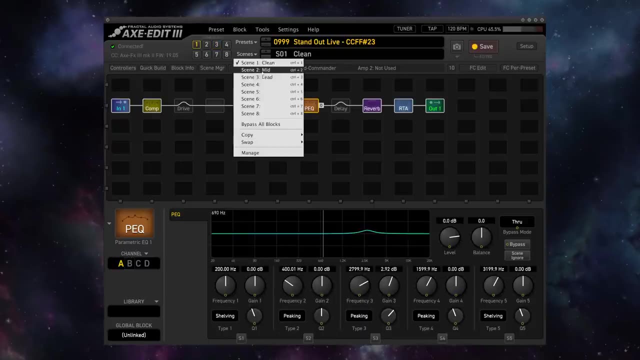 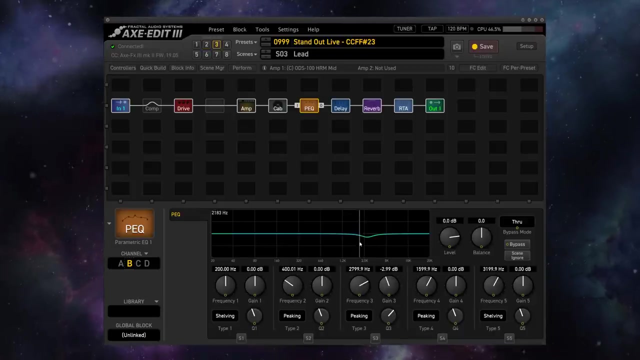 So I'm going to go ahead and, in my clean scene, turn on this boost. in my mid gain scene, turn on this boost and on our lead. keep this slight reduction in pick attack so that my leads are a little more fluid and you hear fewer transients. Okay, so there you have them three. very quick, very 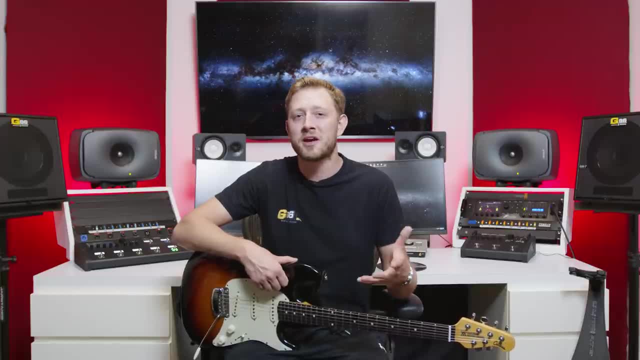 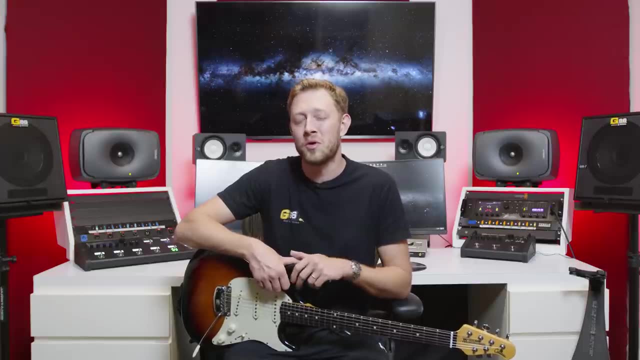 easy EQ tips that'll have you slotting perfectly into your spot in a mix but will also make sure that you are never lost in it. I hope you guys found these tips useful. If you did, please let me know in the comments below what you think and what you've been trying out with your own Fractal unit. Also, make sure to leave. 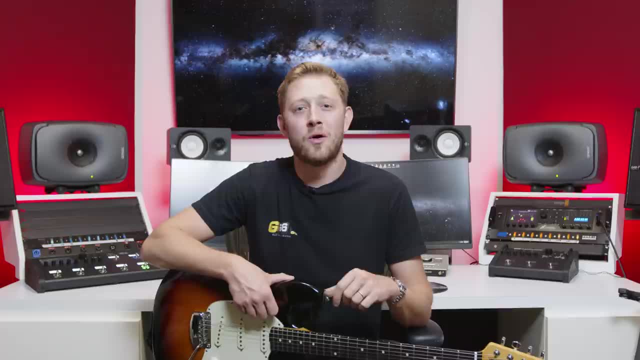 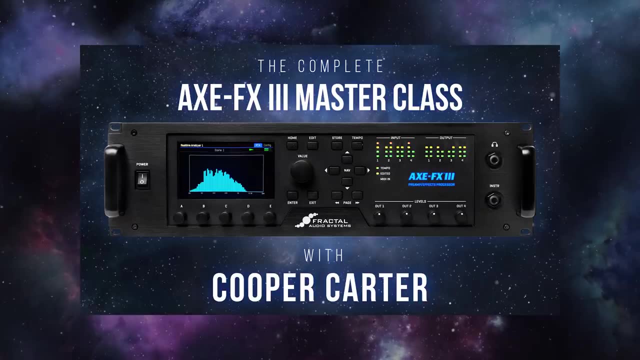 a comment. if you'd like to see something on a future Fractal Friday or chime in on the Fractal Friday forum thread, say that five times fast on the Fractal Audio Systems forum. And if you want to get everything possible out of your Fractal Audio Systems unit, whether that's the Axfex 3,, 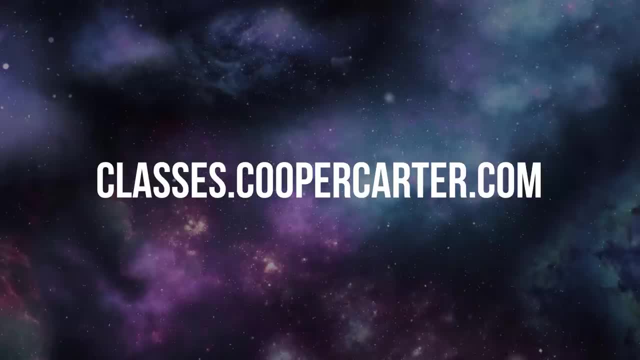 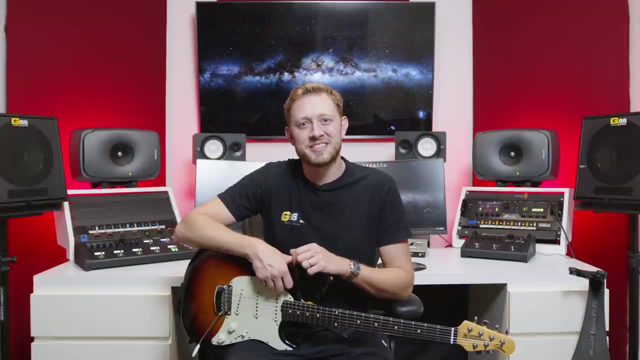 the FM9, or the FM3, visit classescoopercartercom to sign up for my complete master class series For all things Fractal Audio Systems. keep it right here on G66.. Make sure to subscribe. thumbs up this video and, again, leave me a comment letting me know what you'd like to.